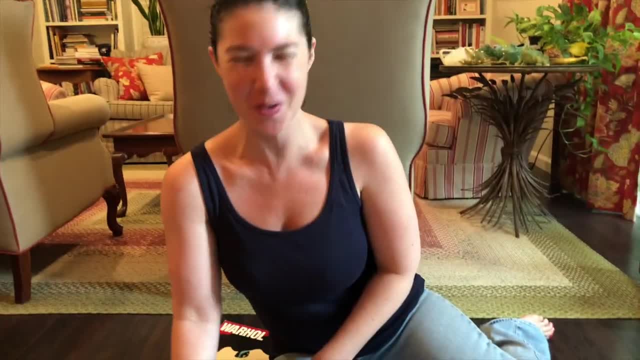 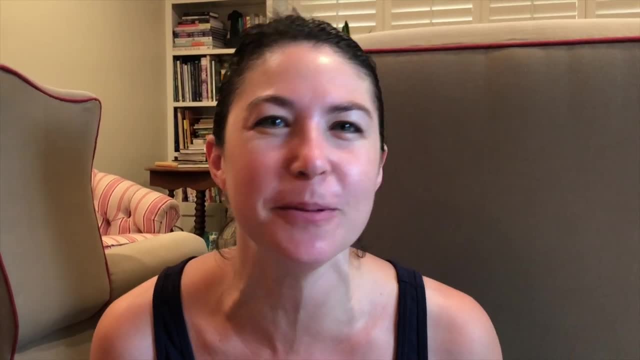 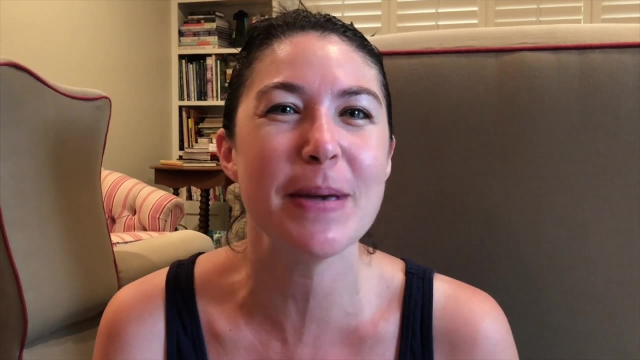 Hi everyone. it's Melissa here, and today I wanted to share with you a little impromptu activity that we started doing last night and we're continuing this morning, and it's a craft activity that maybe you do, something similar to tracing the hands and feet of your child. I'm here just with really 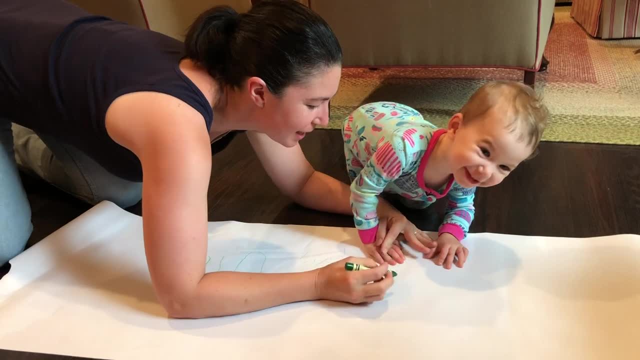 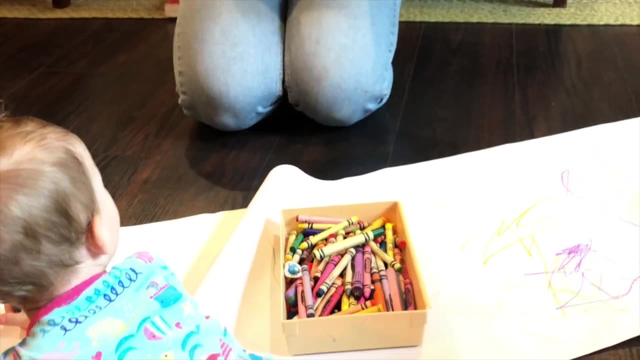 simple materials and a really excited small child, and last night, at the end of the day, she was standing on a long sheet of paper. I just buy those rolls of Melissa and Doug easel paper. They don't actually fit on my easel, so I use them for everything else, like covering the art table or 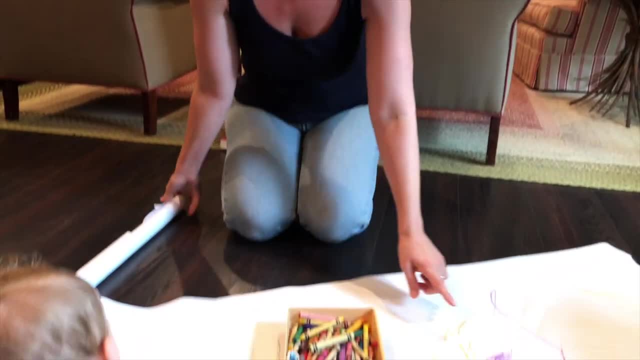 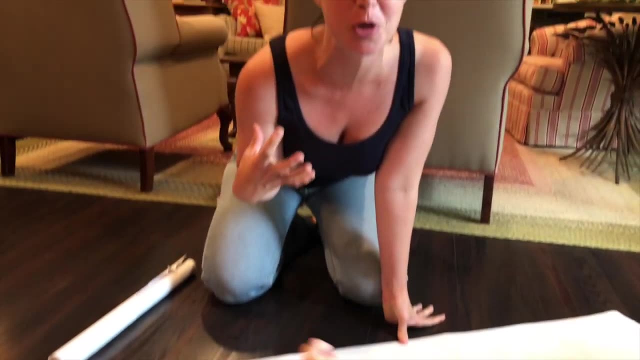 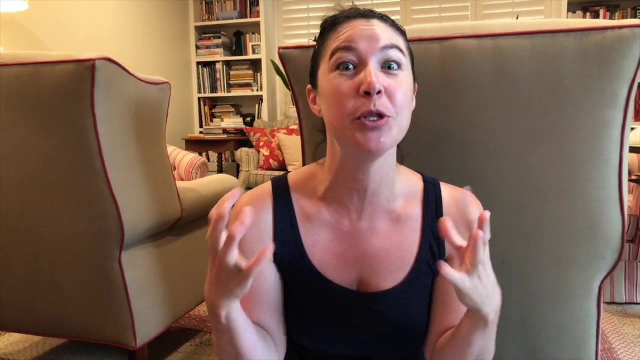 doing art on the floor and we had a lot of fun last night, especially with tracing feet and hands, which I would describe as an activity that's like extra pleasurable for your child because it has that, you know, collaborative element to it, where you're doing art with your child and 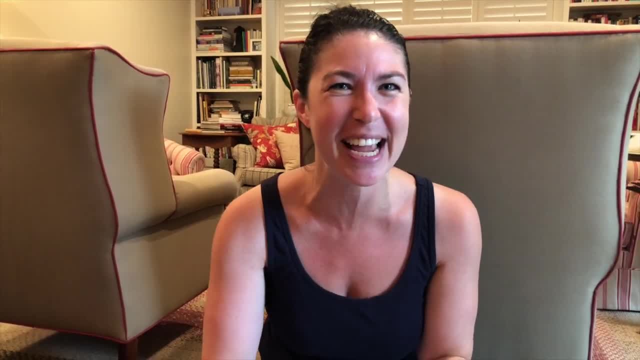 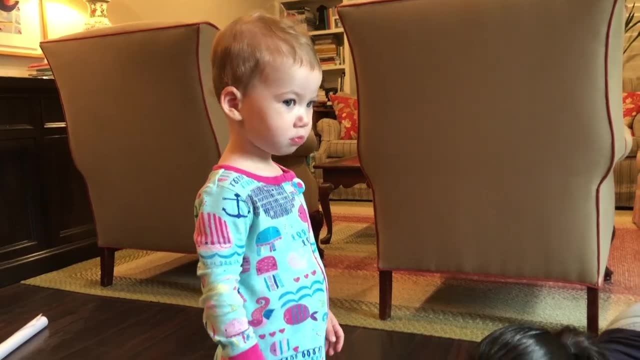 you're touching your child while you do it by holding down their foot or hand, and it was in a weird like massage kind of way, like strangely relaxing for my daughter. The other thing that I found to be really interesting about this- because I have an art background- is that there's 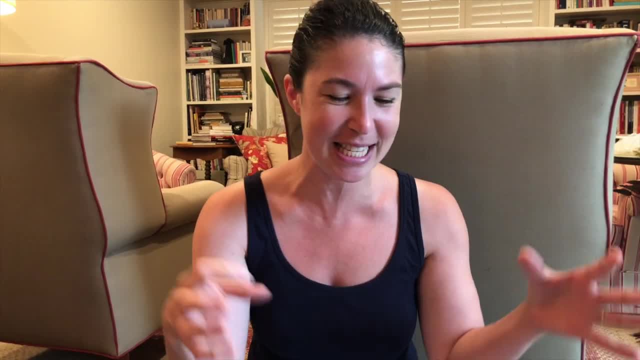 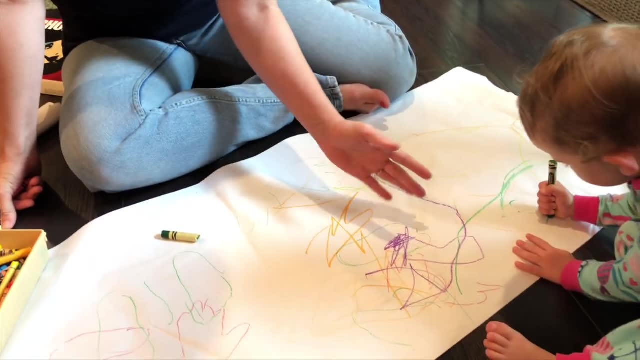 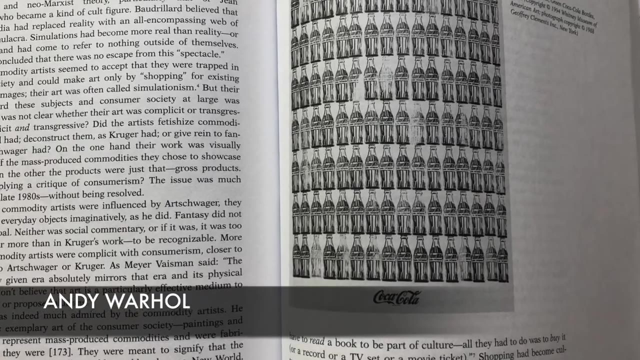 a lot of like art history packed into this. so there is the activity itself and there are techniques used here, like layering and almost like printmaking, where you have a repetition of the same motif in the offset. that is really beautiful to me. There's lots happening over here. This was last night's. 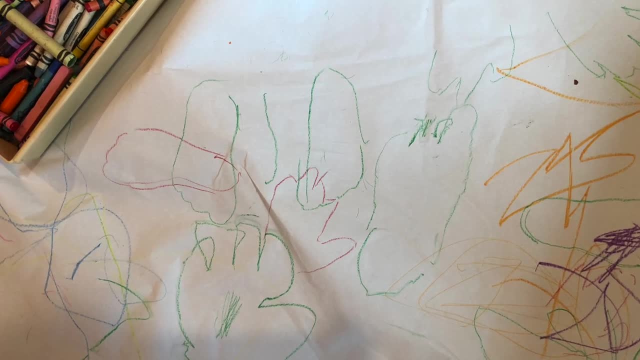 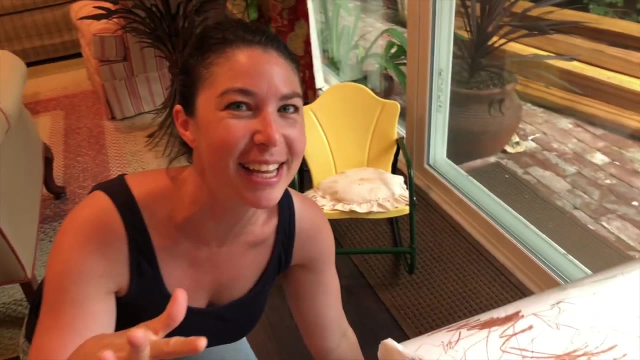 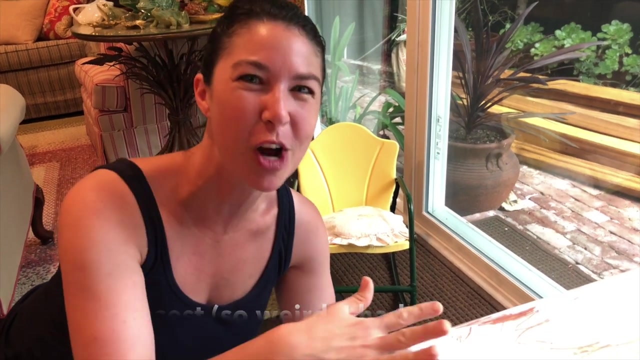 where we had just a ton of layers. In the art technique world this might be called a palimpsest, which is like a literary term of layering, and it's also an art technique term called palimpsest, where you draw something and maybe you erase it and then you draw it again and you get the sort of 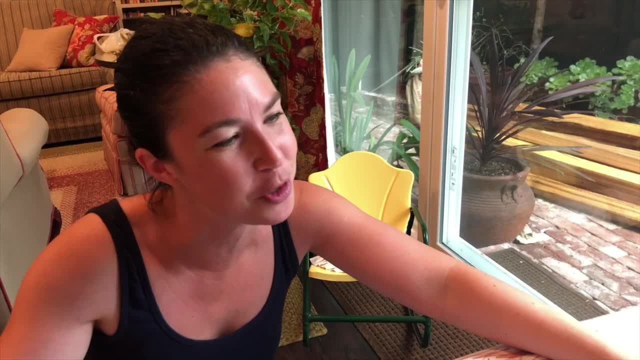 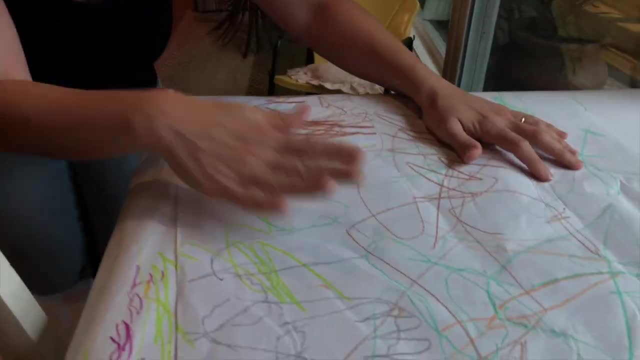 evidence of what was before, and so, from like a sort of higher level art perspective, I find that this is really interesting that my tiny- you know under two years old- child is doing this kind of layering art with me. You can pick up a book at the library.